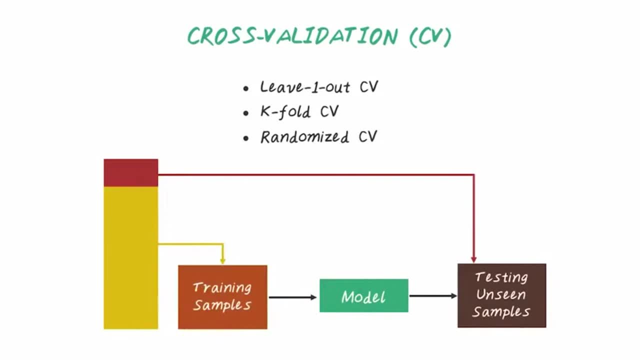 Finally, the performance matrix are aggregated across this iterations, often by taking the average. There are three common methods for cross-validations, namely leave-one-out cross-validation, k-fold cross-validation and randomized cross-validation. In leave-one-out cross-validation we take one example at a time as our validation set. 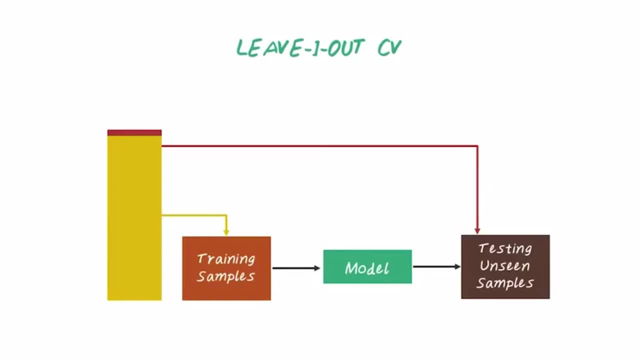 and use the remaining set as the training set, Then repeat this process. Many times goes through the entire data set. The final performance is computed by averaging the prediction performance across all iterations. K-folds cross-variation is very similar to leave-one-out validation. 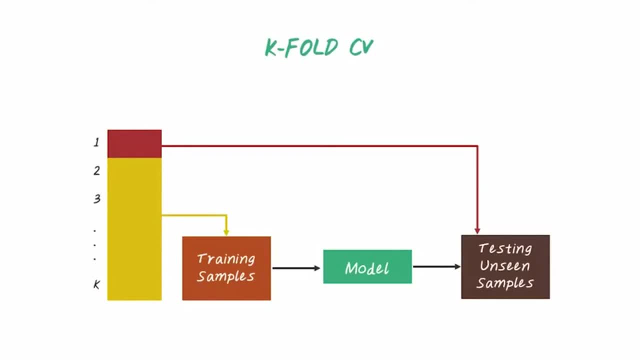 But instead of just using one example of validation set, we have multiple samples in the validation set. More specifically, we split the entire data set into k-folds And we iteratively choose each fold as set validation set and use the remaining set as validation set. 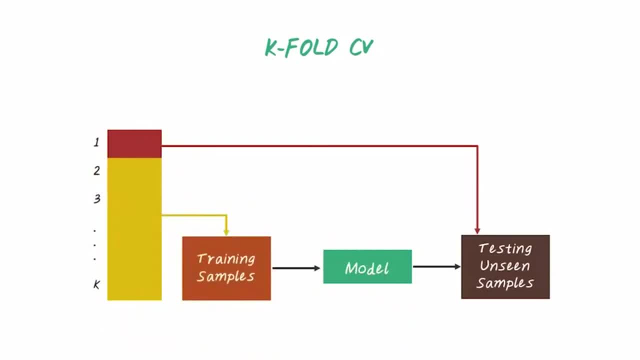 And we use the remaining folds as a trimming set. For example, the fold one would be used as the validation set and the remaining fold will be used as a trimming set to view the model. Then we use a fold two as the validation set. 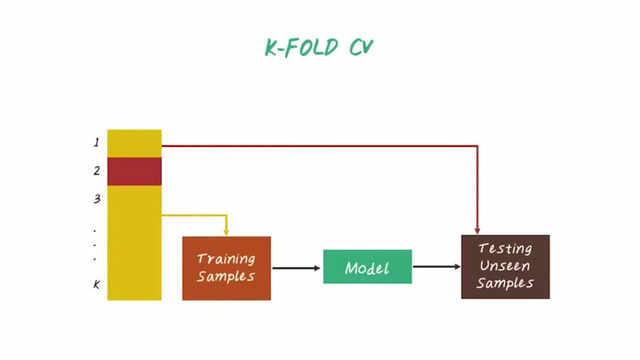 the remaining fold as the training set to be, build another model And repeat this process k times and the final performance is the average over this four different models. Finally, randomized cross-validation will randomly split the data set into training and testing. For each such split, the model is fit to the training data set. 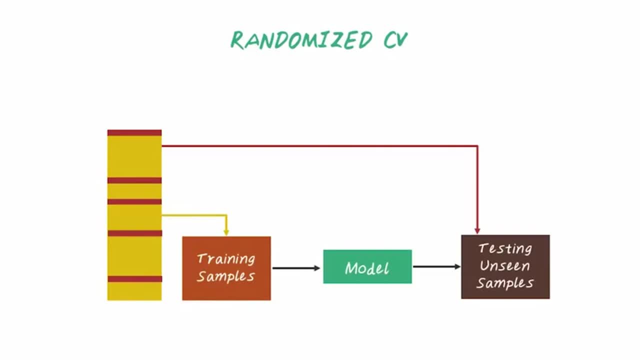 and the prediction accuracy is assessed using the validation set. The result are then averaged over all the splits. The advantage of this method over the k-fold cross-validation is that the proportion of the training and validation set is not depends on the number of fold. 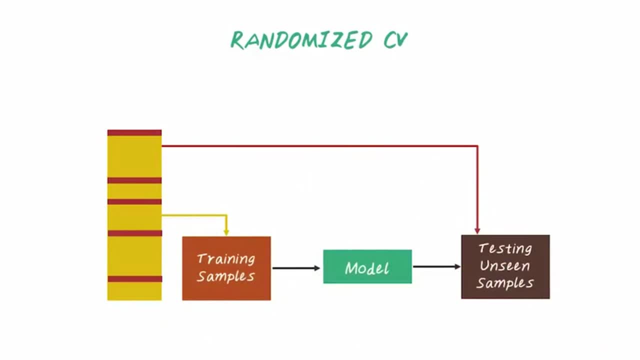 The disadvantage of this method is that some observation may never be selected into the validation set because there's randomization process, Whereas some other samples may be selected into the validation set and some other samples may be selected more than once into the validation set. 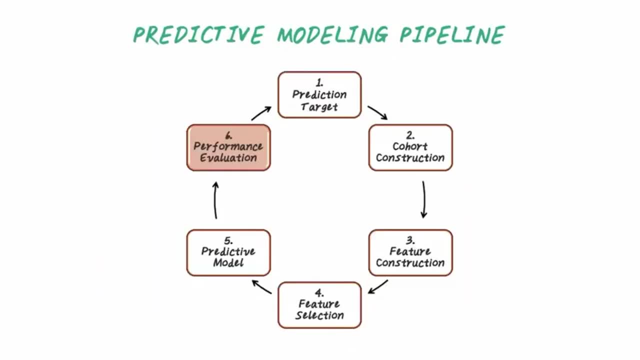 Validation set may overlap. To conclude, in this lecture we introduced the key steps in building a predictive model, which include: define what is the prediction target and construct the right patient cohort. then construct all the possible relevant features from data. then find which features are relevant and view the predictive model. and finally evaluate the model performance.